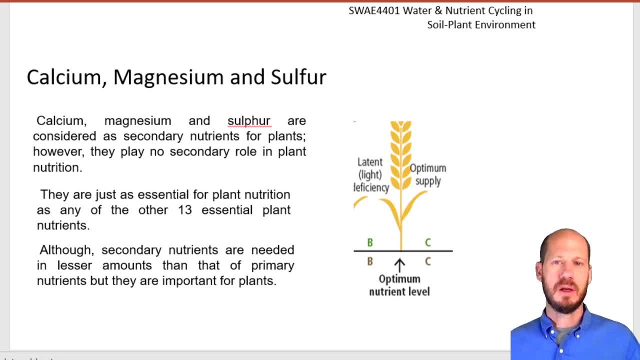 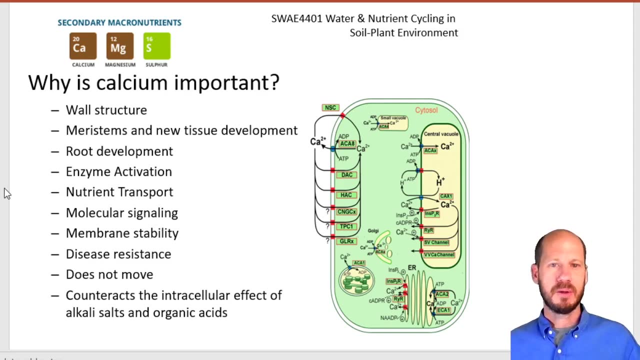 special for, especially for sulfur now, because we don't have atmospheric pollution anymore in acid rains deposit, depositing sulfur in our soils. so why is calcium is important for plants? calcium is important for wall structure, for the, the tissue development, marriage teams, root development, enzyme activation, nutrient transport, molecular signaling, membrane stability. 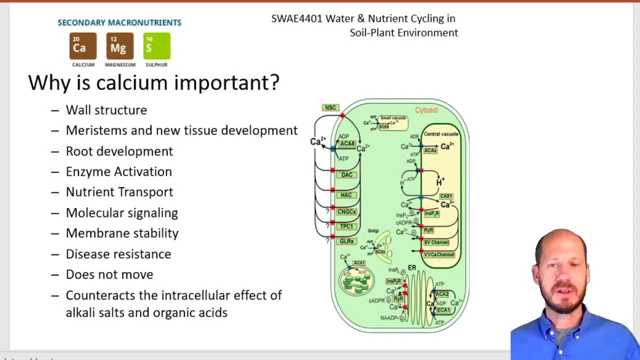 resistance. it's very stable and doesn't- it's not- really well transported in plant tissue and uh, it's actually. calcium is the counter ion that will form the precipitated forms of all the organic acids in intracellular environments and, for example, if the plant produces phytic acid, the, the storage of this phytic acid will usually be calcium. 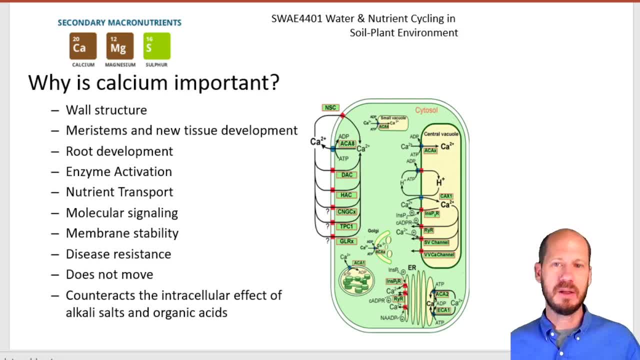 phytate. you know, not phytic acid, but calcium phytate. so calcium is, whereas potassium is always the go-to ion for soluble uh, uh to be the counter ion in soluble forms. when you have to store this nutrient in precipitated forms, these are usually being uh contracted by calcium, and calcium is. 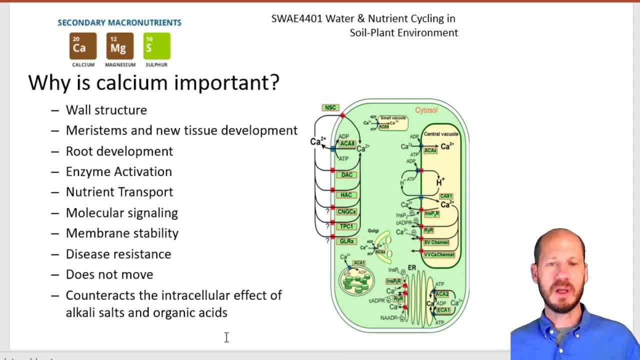 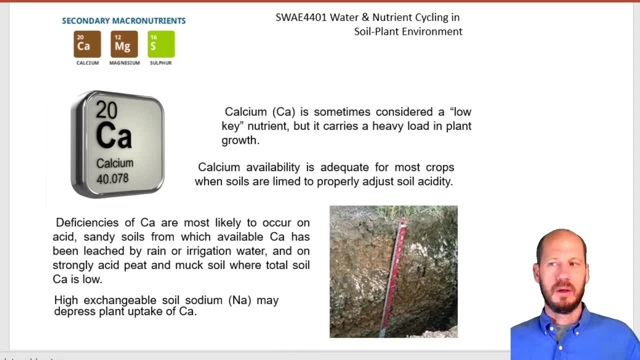 important for regulating this um uh contracting the, the negative charge of the organic acid in the cells. so calcium is usually considered an element of smaller importance. the the important. the smaller importance is usually due that we have a huge amount of calcium in terrestrial environments, so because of that it's very uh hard to find situations where calcium is so deficient. 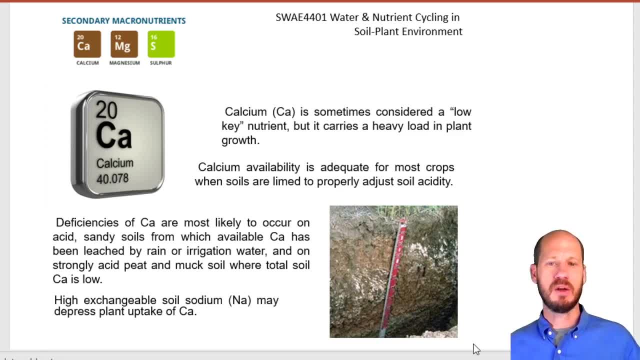 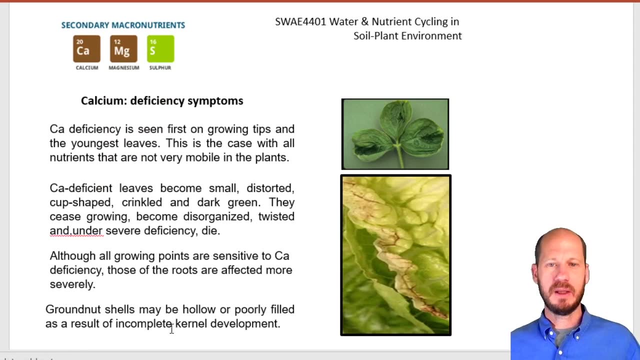 that you will need the calcium fertilizer application in order to have an adequate calcium nutrition, but nevertheless, we can find the situations even in high calcium soil. so I'm going to explain this in a little bit. so one of the main things about calcium: when you, when you identify that you have a 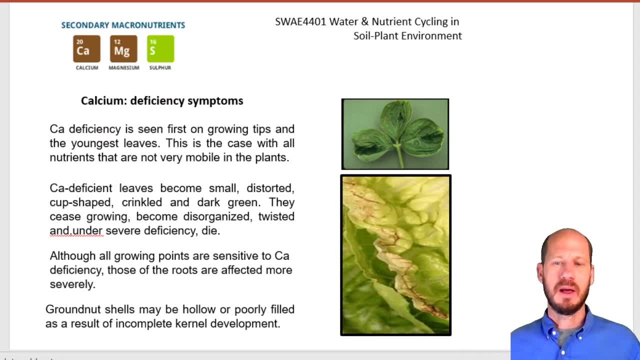 calcium deficiency is. you have the leaves of the plants are curling. you know they're curling and bending in themselves, like they are trying to make like a round shape and you know, picking up it together like you see here in the photograph, you know. so this is very typical and you will see that in, in, in. 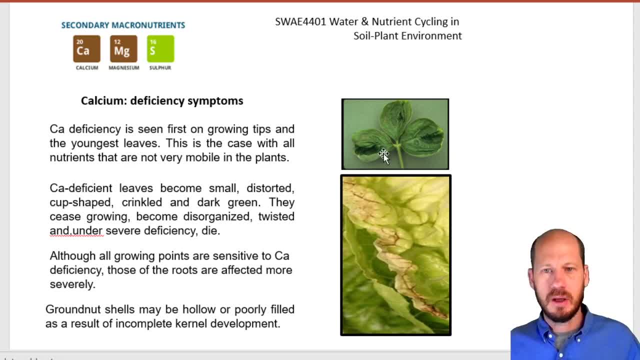 tomatoes, potatoes, beans. there's dicotyledons mainly. you will see this behavior where the plants are curling on itself and this is the symptom of calcium deficiency. yeah, trying to grow, but there is not enough calcium in the leaves of the plants. so you can see that the leaves of the plants are. 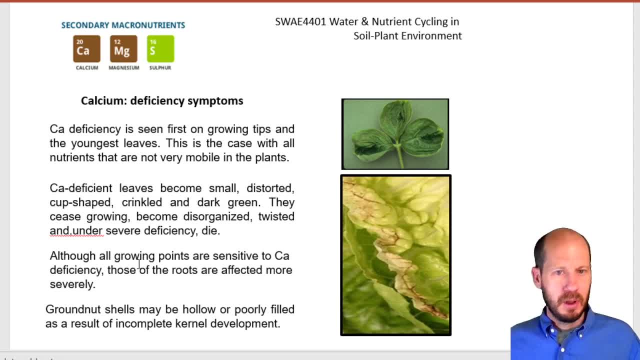 growing and the calcium for promote this. she wrote. so this: sometimes you can confound this for these symptoms with other, with other problems of the plants, for example salinity, but usually when you see the curling of the leaves, that is when you will have calcium deficiency, so the calcium cycle will be more. 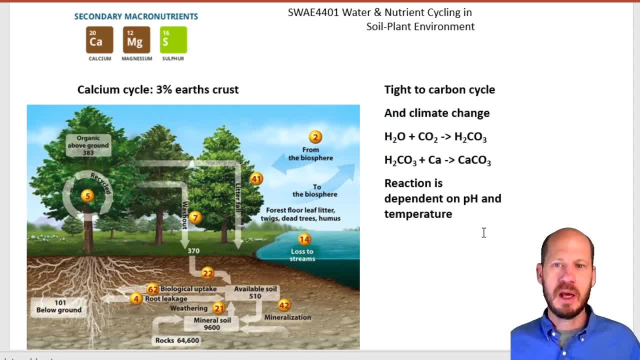 similar to what is the phosphorus cycle in the potassium cycle. you usually don't have any atmospheric component of this cycle. it's usually coming from the rocks and in the water and it's being cycled into the plants and into the soils and being decomposed or in cycle from through the organic matter, yeah, and until it's lost. 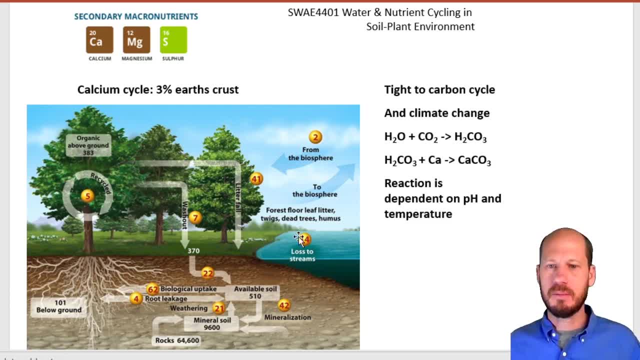 and reached the waters. there is one big thing that we have to mention about calcium is that the calcium cycle is very tightly linked to the carbon cycle. the reason being is because the co2 dissolved in water forms carbonic acid. in the carbonic acid reacts with calcium and for it forms. 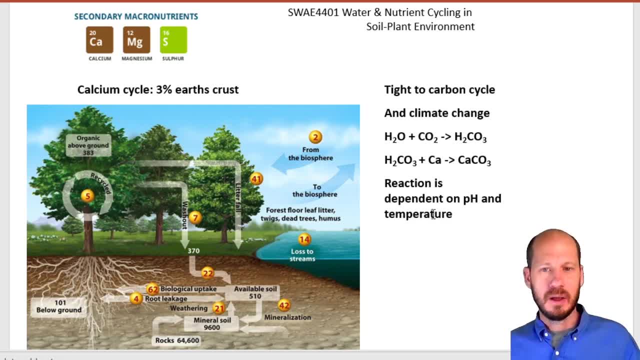 calcium carbonate- all this white material that you will see on in sediments and soils, and it tends to be carbonates the are precipitated on the soil. So the calcium carbonate is a very big forms of calcium storage on the soil. They're usually very unavailable to plants and this is one of the reasons why you can. 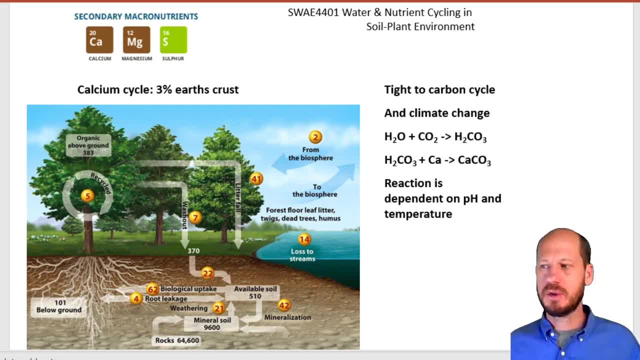 find in Oman calcium deficiency in some situations because even though you have sometimes 30 percent of calcium carbonate in the soil, the calcium carbonate will represent a form of calcium that is insoluble. in many times You need to acidify the soil in order to release the calcium by 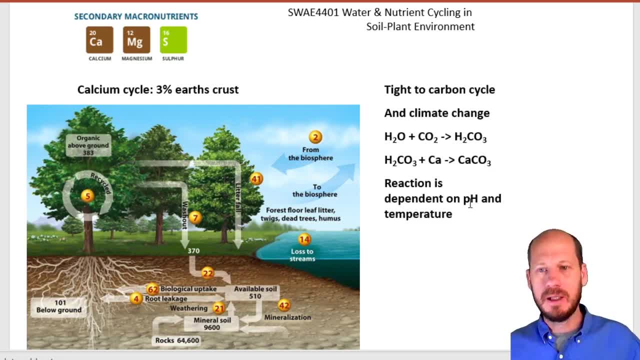 emitting CO2 from the soil and sometimes the alkalinity of the soil is so high, especially when you have sodicity problems and this alkalinity when it's too high and the plants are not able to counteract this alkalinity By using only root exudates and if they are not able to acidify, the rhizosphere. 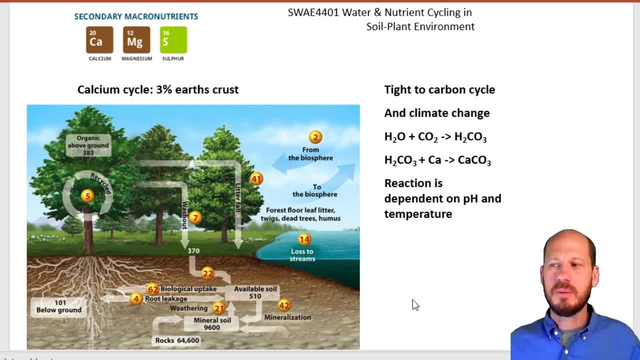 to release the calcium, then you might have a calcium deficiency, even if you have a soil with about 30 percent calcium carbonate. So you have, might have, a huge amount of calcium in the soil and even though, even then you might have calcium deficiency, depending on the situation. 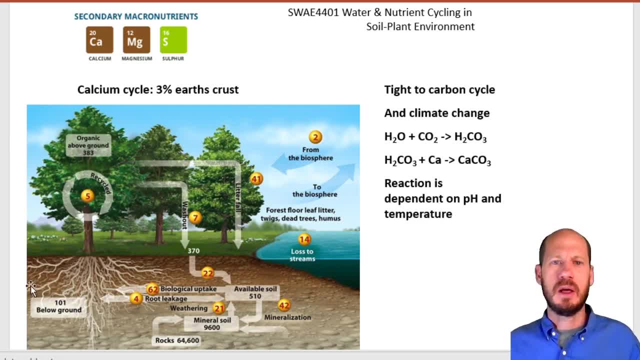 But in general, overall, around the globe, calcium represents three percent of the earth's crust, so in general, you will have enough calcium for nutrition, and very specific cases is where you will need to apply calcium for for plant nutrition, and when you do need it, the form that you apply is by using lime. So whenever 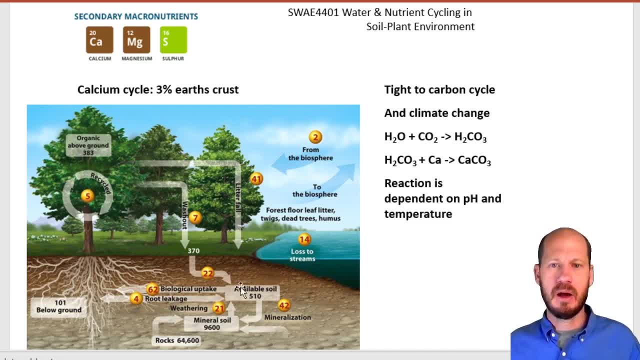 you have very acid pHs and you already leach the calcium from the soil because of the acid pHs. when you use the lime to correct the pH, you are already applying calcium, so in that way you don't have to worry about calcium nutrition when you are correcting the pHs of the soil In very alkaline. 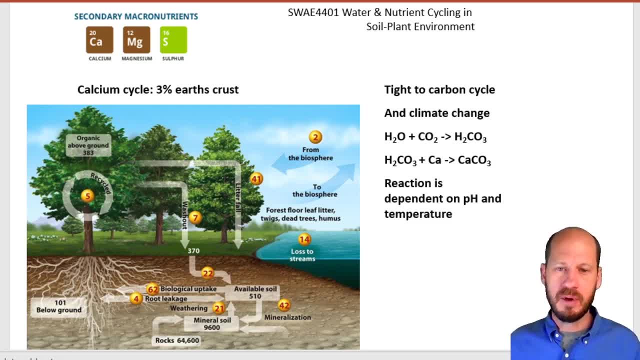 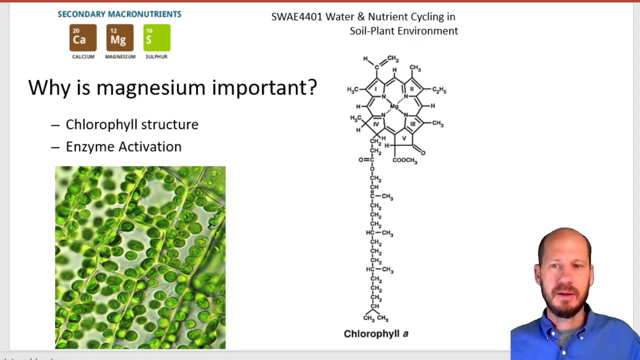 pHs, then you will usually have a huge amount of calcium in other bases also. but the main problem will be when this calcium is very insoluble- The case for magnesium in the plants. although magnesium has a similar behavior in soil, it forms alkaline precipitates. 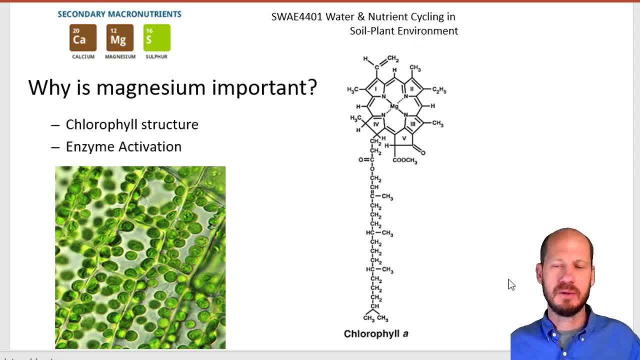 it behaves very similar to soil. it's very abundant in in solid systems. The role that magnesium has inside the plants is very different from the one that of calcium. Magnesium is part of the chlorophyll structure and the magnesium on the center of this chlorophyll structure head. 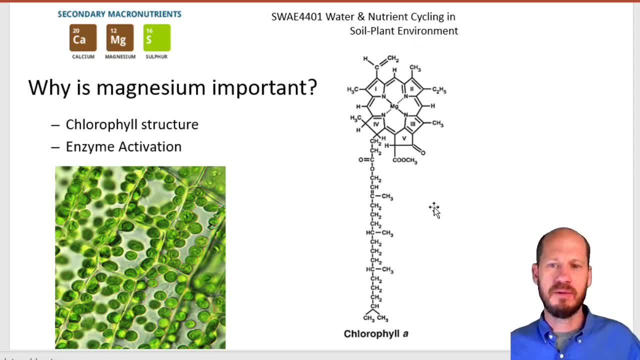 is what is able to absorb the wavelengths of light and vibrate these molecules and this is what allows the photosynthesis to occur. so magnesium deficiency is directly affecting photosynthesis, yeah, whereas calcium deficiency is usually affecting tissue growth. but magnesium, this, its unique role, is on the chlorophyll and the photosynthesis. 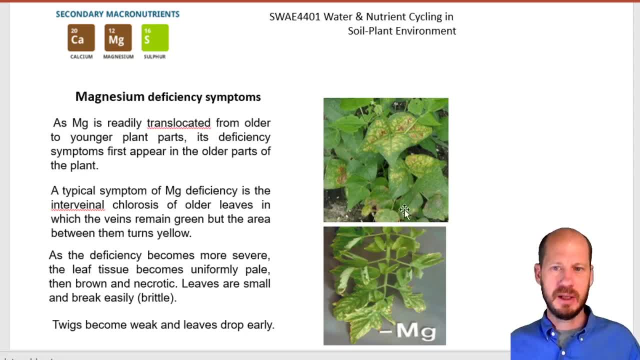 So the magnesium deficiency? it tends to look a little bit like what you see for potassium and you have this intravenous chlorosis because, similarly to potassium, the magnesium can be transported. you know, you can transport magnesium from old leaves to new leaves. so whenever you have deficiency, the plants will try to deplete this magnesium and bring it to new tissues and that's. 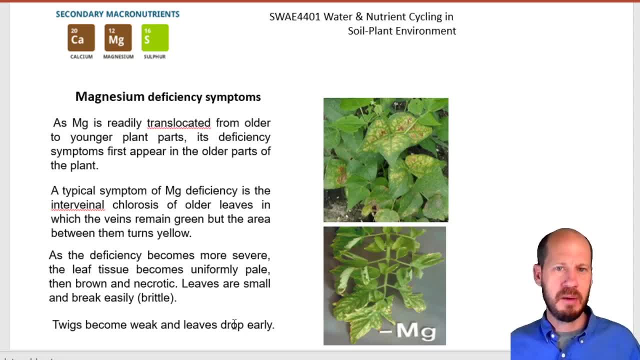 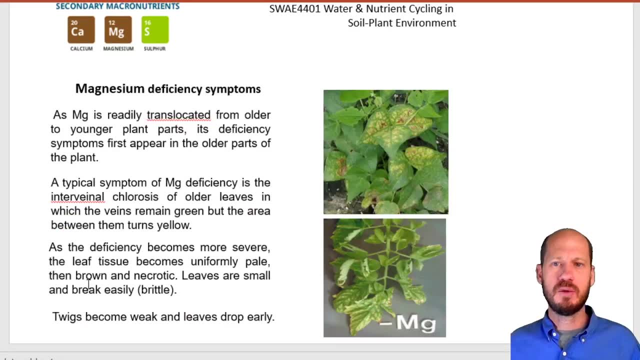 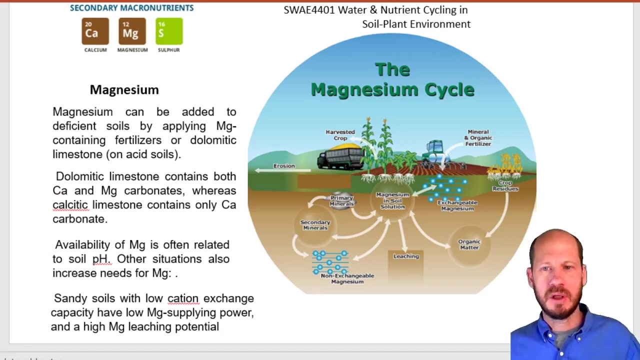 why you see this deficiency, intravenous chlorosis, happening. yeah, with magnesium, very different from the symptoms for calcium also. so chemistry in soil is very similar to magnesium and calcium, but the the behavior in plant tissues and the symptoms in plant tissue they are radically different. so the magnesium cycle, as i was saying, is similar from calcium. yeah, you, it will not have. 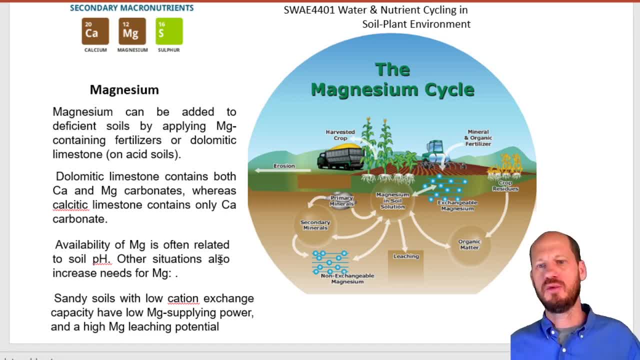 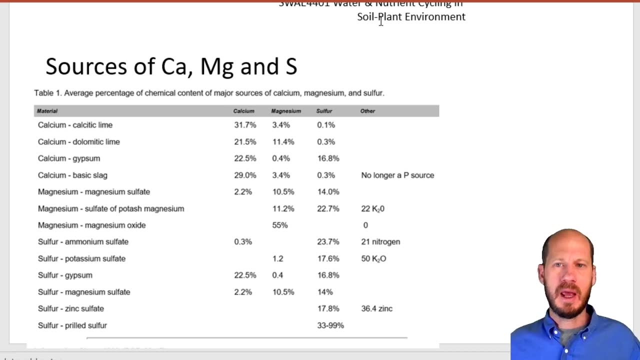 an atmospheric component. it's been cycled through the rocks into the soil and in the soil it's been taken and deposited on the soils and cycled, and then it's leached or lost through waters. The main sources that you will have for nutrition of calcium and magnesium they will be limes. yeah. 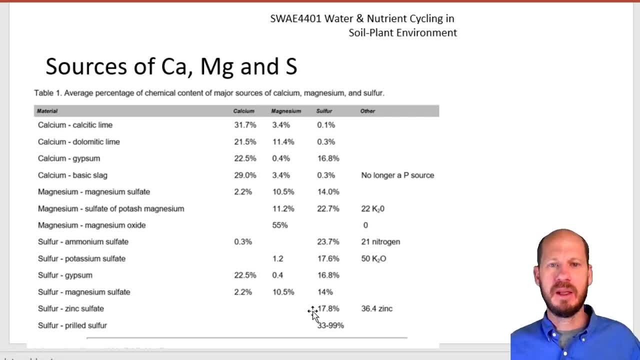 so a calcitic lime, dolomitic lime. they are the main sources of supply of these nutrients to plants. the magnesium water that we have combined with even sulfur, like gypsum, calcium sulfate is the main form of that. you apply sulfur to the soils and you have many, many other combinations: magnesium. 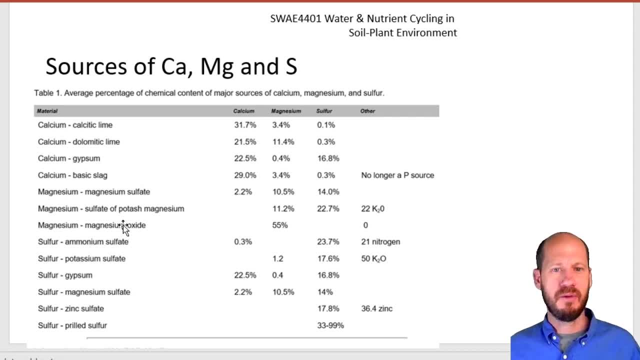 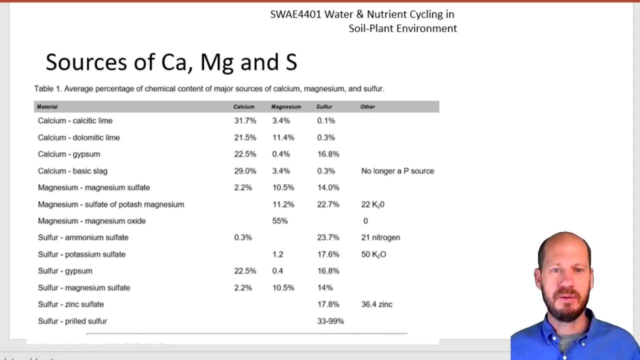 sulfate um magnesium, oxides of uh, sulfate of potash magnesium. there is actually a variety of different fertilizers that contains calcium magnesium in the soil. so there is a variety of different fertilizers that contains calcium magnesium in the soil, sulfur, but the main ones will be calcitic and dolomitic limes. so actually, 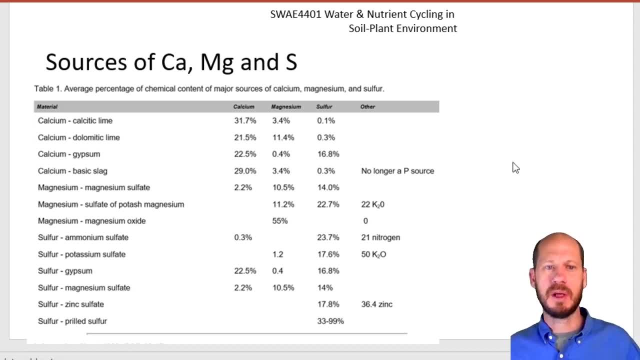 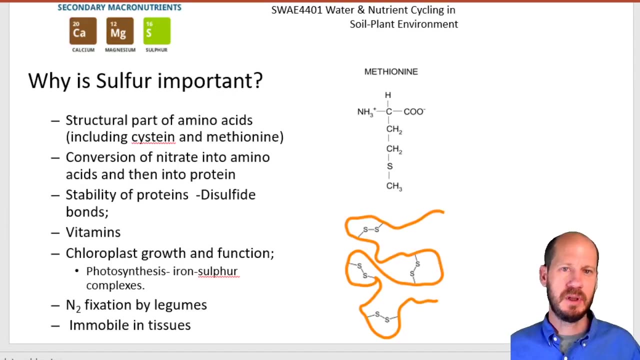 the will. you tend to expect more calcium and magnesium deficiency when you have low pHs, and by correcting the pH right away, you will have that. you already using enough calcium and magnesium as fertilizers. sulfur, on the other hand, is a completely different story. sulfur, it's raw in plants, is mainly 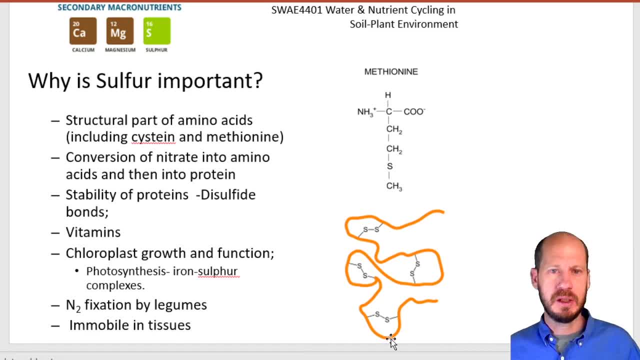 because it's part of amino acids and proteins. so the behavior in the plant is similar to the nitrogen in the way that the nitrogen, the bulk of the nitrogen in the plants or in the protein molecules. similar that will be for sulfur, just the only difference is that the for the sulfur it's a completely different story. 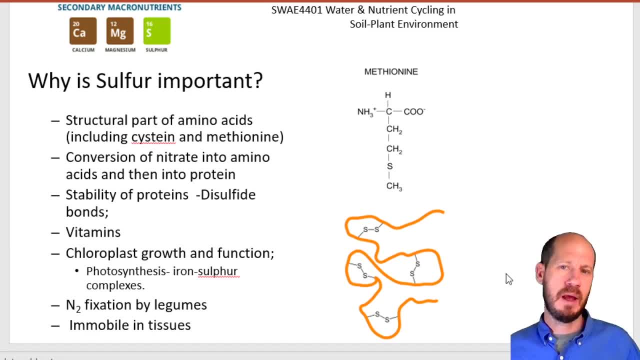 sulfur you will have a lower amount than you will have for nitrogen, so you need less amount of sulfur than you have for nitrogen. but you will have a similar behavior in the plant and also in the soil in the sense. I will explain a little bit more about the behavior in the soil, but sulfur is hugely important. 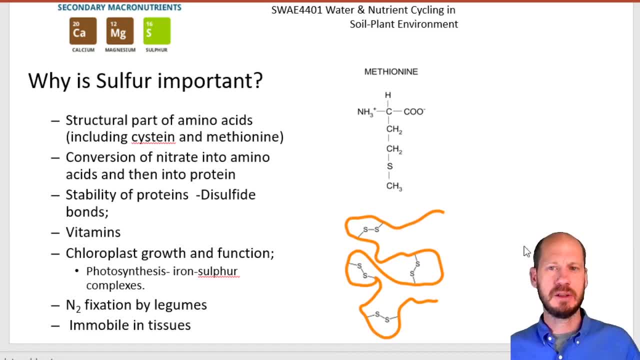 in different processes that are regulated by these proteins. so every protein that contain either cysteine or methionine will have sulfur and the sulfur in the proteins. it's very important for the stabilization of the structure of these proteins because the sulfur can form desulfide bones and 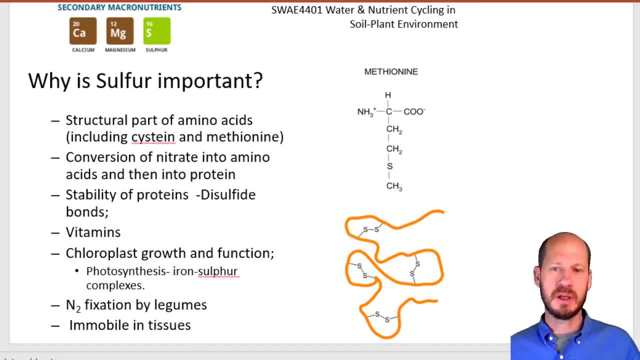 therefore, the structure of these proteins becomes a little bit more, a little bit more rigid and allows the proteins to have more stability and do not lose the activities of different enzymes in different conditions. so the strategic location of this desulfide bones on the protein allows for having the formation of three-dimensional structures on these. 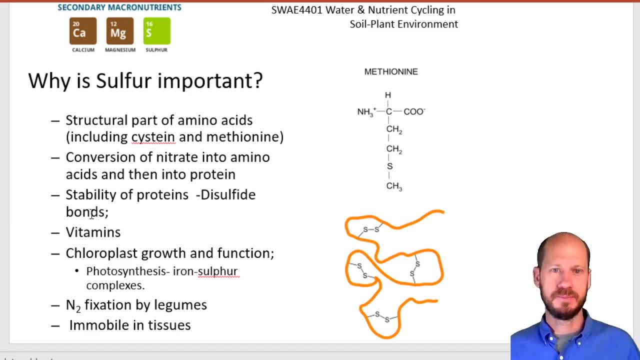 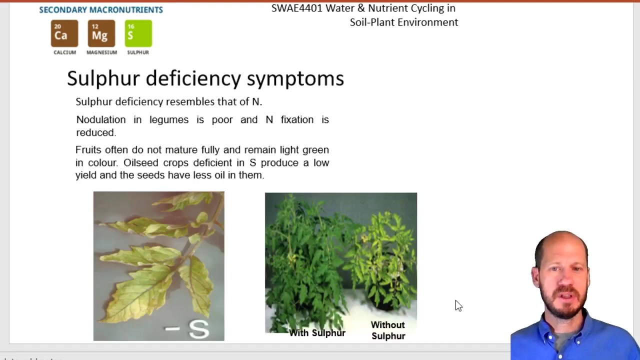 proteins, which are hugely important for their function. okay, so sulfur is part also of vitamins and is very important for chloroplasts and plant growth function. nitrogen fixation by legumes also is highly influenced by sulfur nutrition and sulfur is not very mobile and plant tissues the symptoms of sulfur deficiency will be yellowing. yeah, like. 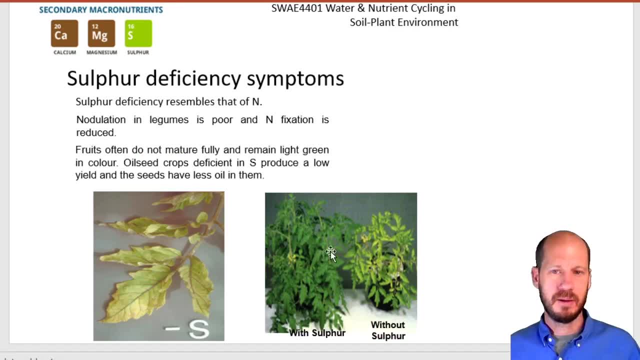 nitrogen, because it's like. the reason is because you cannot produce enough proteins and then, therefore, you have this yellowing of the leaves. yeah, so this is why sulfur is similar even to, yeah, how it looks like on the plants. the leaves are also yellowing. yeah, so this is why sulfur is so different from. 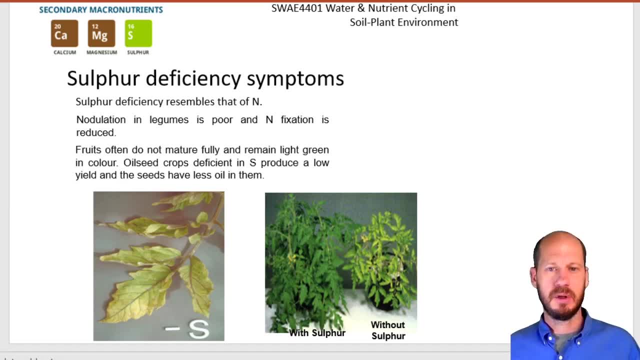 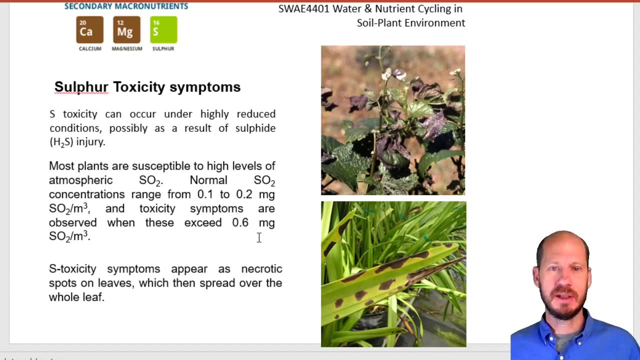 nitrogen. in terms of the toxicity of nitrogen, the the fruit maturation also it's. it's very dependent on sulfur, different from nitrogen. you can have sulfur toxicity symptoms. yeah, you can have sulfur toxicity, but nitrogen also. you might have ammonium toxicity. so it's kind of in the same ballpark of of. 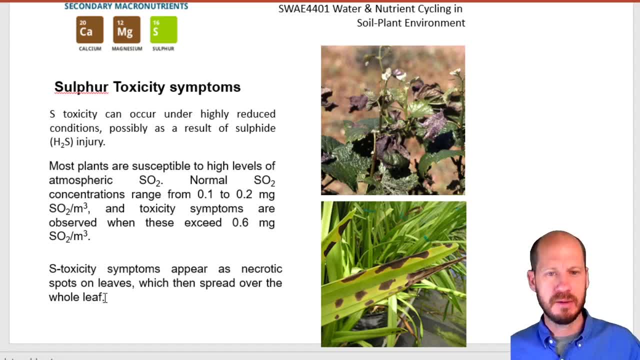 um nitrogen will have more physiological roles than sulfur because it's involved also in DNA and RNA, but similarly you will have a sulfur toxicity if you have excess sulfur applied. usually that is when you use excessive lead fungicides containing sulfur. otherwise it will not cause toxicity. usually you would not. 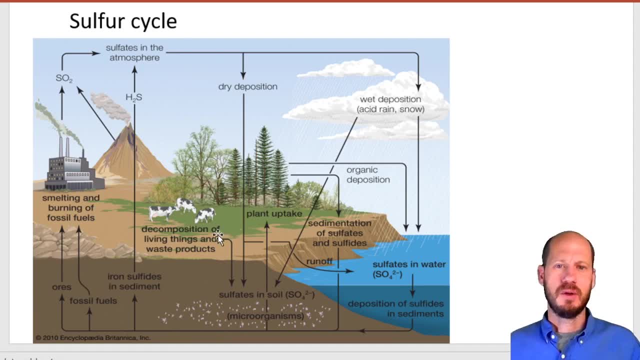 find toxicity. sulfur cycle is very complex. I will not detail completely and one of the the main things that you will find on the sulfur cycle is that it's heavily dependent on microbial transformation. of this, I have a lecture on soil microbiology course which details all the microbial processes. 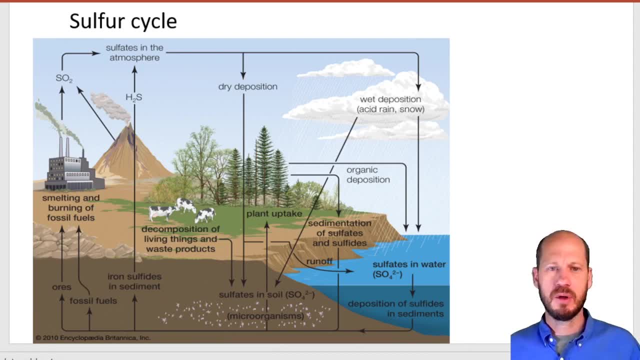 on the sulfur cycle and if you want to know more about all the transformations in the sulfur cycle, please go for that lecture in the playlist of environmental soil microbiology and then you will see all the different bacteria that is, or they are, influencing this. sulfur transformations in anoxic and oxic environments. but mainly you will have that sulfur will have a heavy 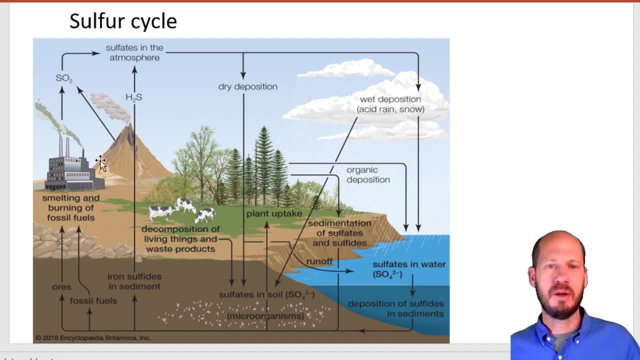 atmospheric component, either by atmospheric pollution through the burning of fossil fuels or by volcanic activity, or by bacteria. they are reducing sulfur and emitting hydrogen sulfide. so this atmospheric sulfur can be deposited as in soils by acid rain and can be uptaken in cycle in the soils in the 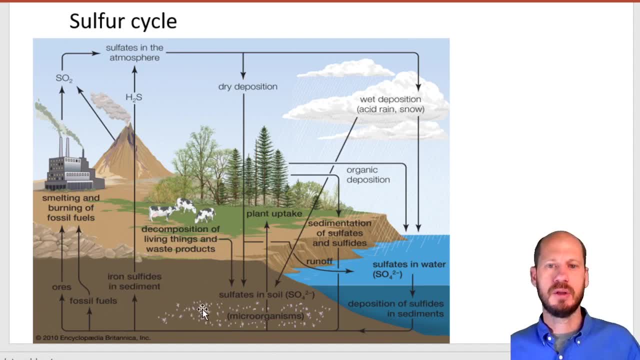 plant tissues and decompose, similar to the nitrogen, you will have. the most of the sulfur in the soil will be present in the organic matter. so if you have low organic matter you will likely have low nitrogen and low sulfur. so in the in waters of soul this sulfur will have their own cycling through. 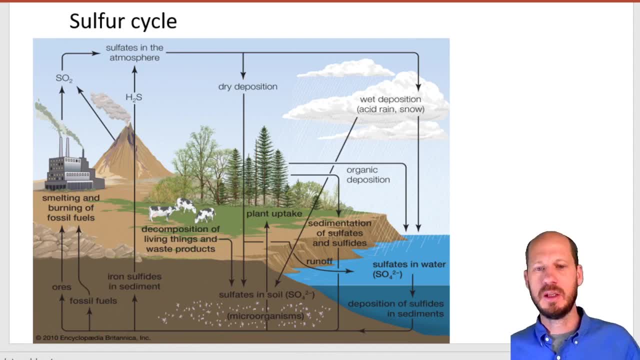 different organisms and will go through different processes of reduction and oxide oxidation, either as a source of the nutrient, sulfur, but also as a source of energy for different cumulative trophic microbes. these chemolithotrophic microbes are also present in soils and they're very important. 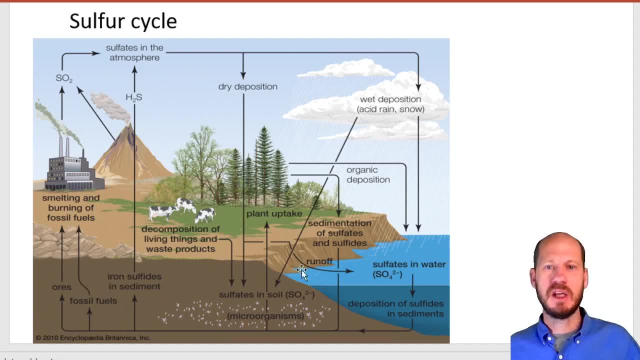 also for the dark carbon fixation, because these are autotrophic microbes. so i would not go very deep on what is the microbiology of the sulfur cycle. but please, if you are interested, go in the other lecture, um in the environmental soil microbiology, and that will be explained in detail. 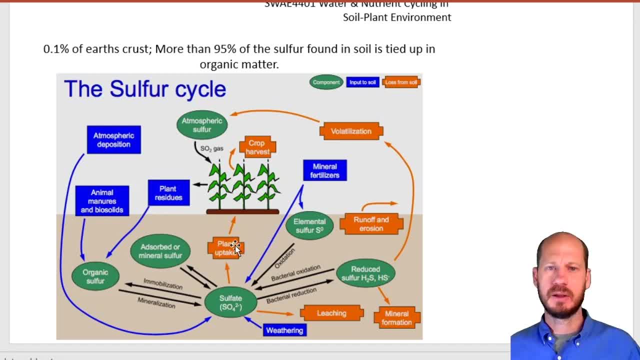 what we are really interesting now for the, the, the sulfur- for this uh lecture is about what is the implications of its chemistry for plant nutrition and what should we do about it. okay, so actually the main source, the main pool of the, the sulfur in the soil or organic- is organic sulfur. you know, the main pool of sulfur in the soil is organic sulfur. 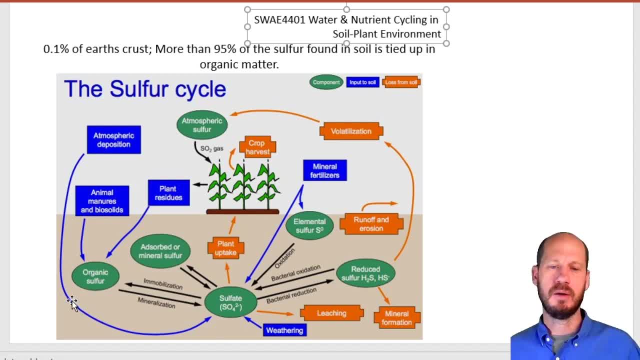 and this is being immobilized by microbes and plants in the inorganic molecules and mineralized by the microbes into sulfate. some of the sulfate, if you have reducing condition, can be transformed into elemental sulfur or be emitted to the as a gaseous form to the atmosphere. 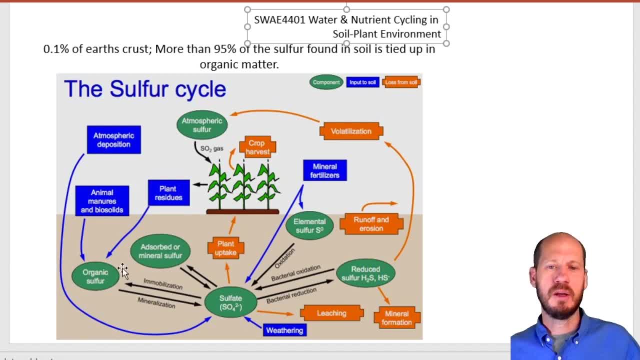 as hydrogen sulfide. the sulfate molecules can be also leached and the sulfur can be taken off by this from these fields, through plant tissues, uh, and also, uh, by erosion. yeah, so if you have, if you're concerned about the level of organic matter that you have on your soils, 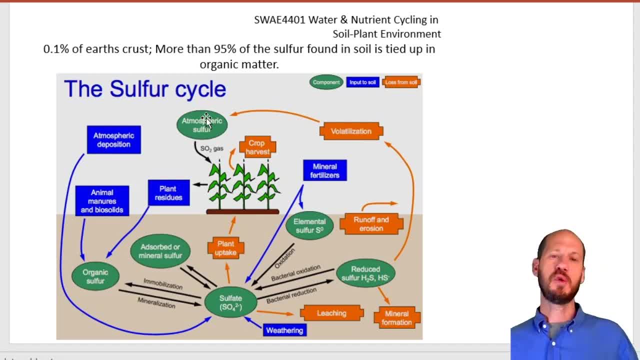 and if you want to replenish the organic matter in your soils, most likely you have an sulfur for plant nutrition because they will be coming from the uh, the, the hydrolysis of the, the, the proteins on the, the, the plant residue can be lost. so 258 00F will be lacking a little bit on the organic matter that you have on your soils. most likely you have enough sulfur for durum nutrition because that will be coming from the uh, the hydrogens of the, the proteins on the, the, the plant residues, and they will come from the radiolysis you have from the Yoshiro and lifestyle uh. that, even though it has more 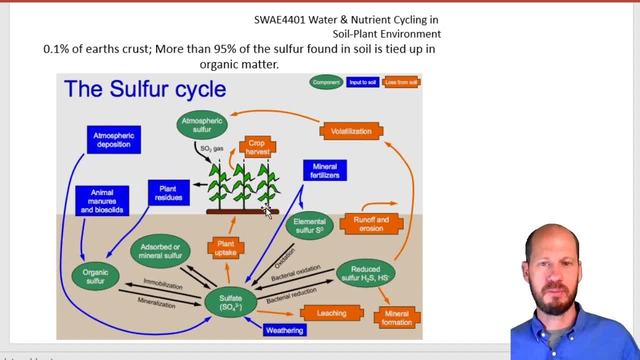 the hydrolysis of the, the proteins on the, the plant residue and the organic matter that you're adding. that will come enough sulfur for plants, for sure, but there are other ways that you can supply this for plants, and one of the ways is through elemental sulfur or gypsum calcium sulfate. 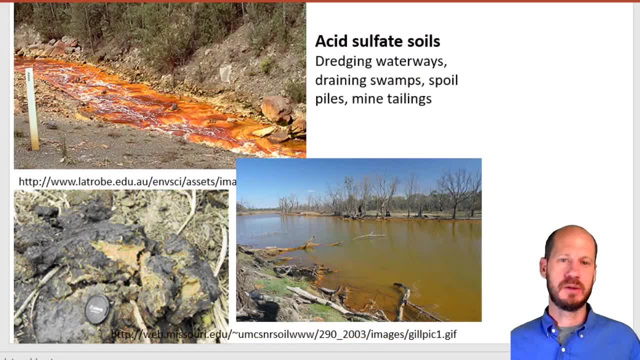 in acid soils, sulfur can be a problem. yeah, sulfur can be a problem in acid soil. so what happens is you if you have excess sulfur. this sulfur tends to take the form of sulfuric acid. yeah, is the sulfate when it's compensated by hydrogen is sulfuric acid. so in these situations in acid, 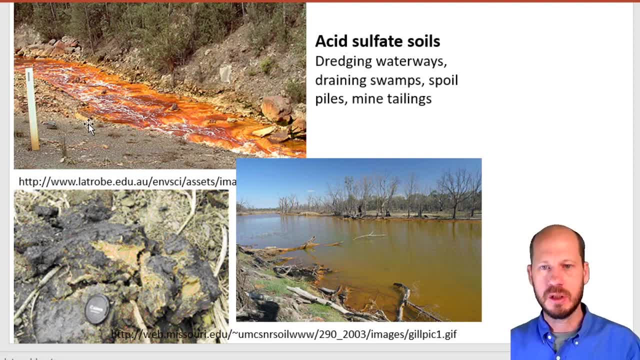 soils. they're usually in tropical regions, uh weathered soils with high rainfall. if you have that, this, this is excess sulfur that's happening on the soil. the sulfuric acid will dissolve the iron on the soils, which the soils contain- a huge amount of iron. there are oxy salts in general, and 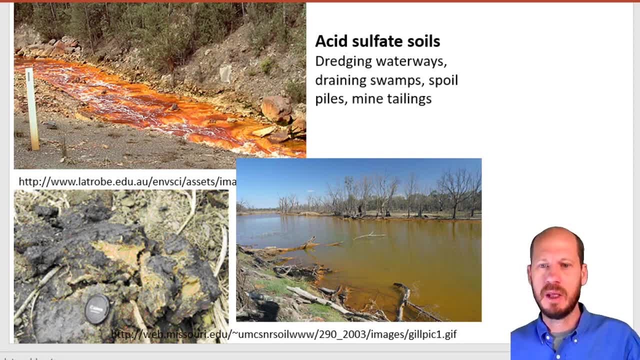 excess sulfur will dissolve the irons and these irons will be a huge contaminant of waters. so you will see this water courses that can be heavily contaminated by this dissolved iron is. this is due to the excess of sulfur that can come from mining or volcanic activity or any other source of. 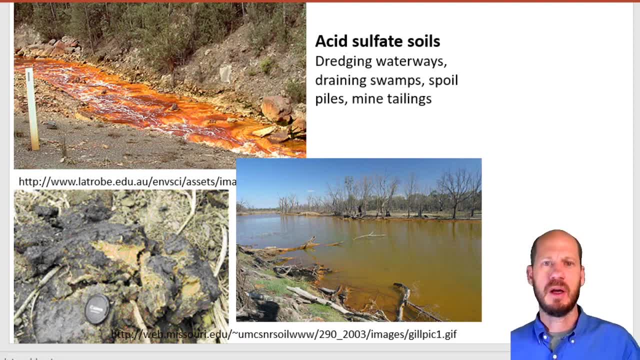 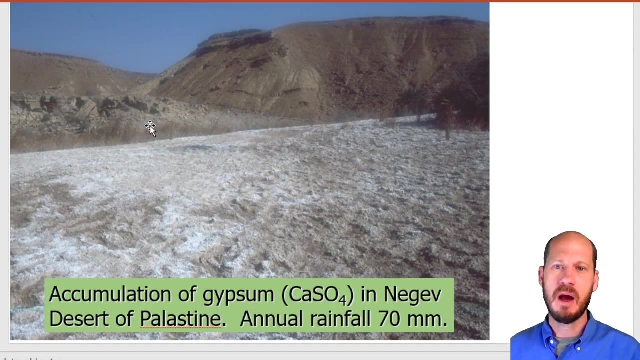 contamination of sulfur can be a big problem for uh acid soils. where you can, we can further acidify and dissolve the iron on on this uh situation. but this is not the case of a man or man is usually the case of having very alkaline soils and you will have minerals, namely gypsum, in the soils. 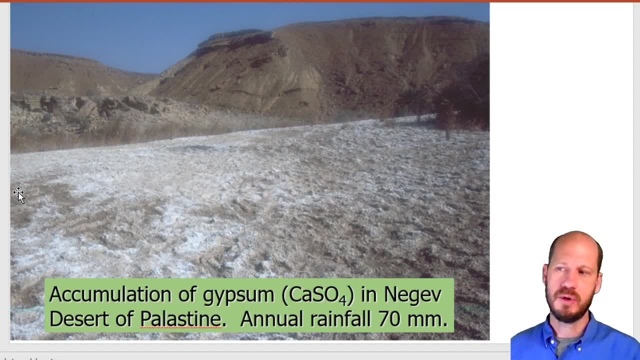 that will be accumulated in organic sulfur. so you might have in alkaline soils like the ones in oman. you will have the possibility that you will have not only sulfur in the organic matter but a lot of sulfur locked in in organic forms like calcium sulfate. uh, and this calcium sulfate. 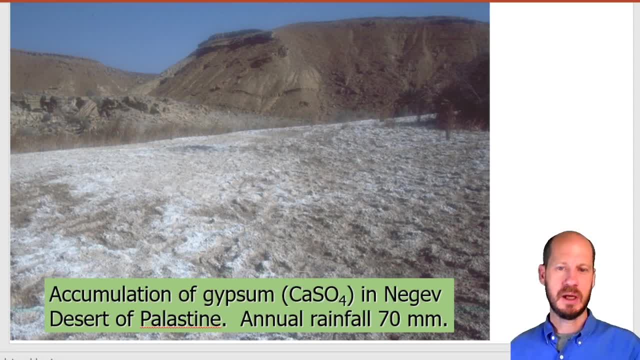 you can have huge deposits like you're showing in Palestine, but in Oman it will be part of the soil minerals. you know, like you have carbonates, you will have some gypsum also in these systems. this is very typical. when you have also seawater intrusion, you will have that. the soils will contain more. 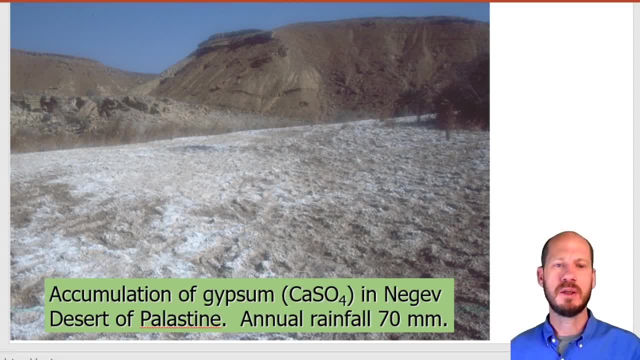 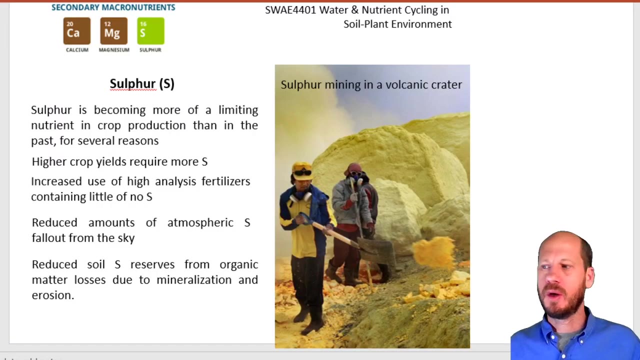 sulfur than the other soils, because the seawater will have some amount of sulfur that will be added to the soils. also, where did the sulfur come from when you add them for fertilizer? the sulfur is usually mined in the past or mined for volcanic deposits of any creatures. 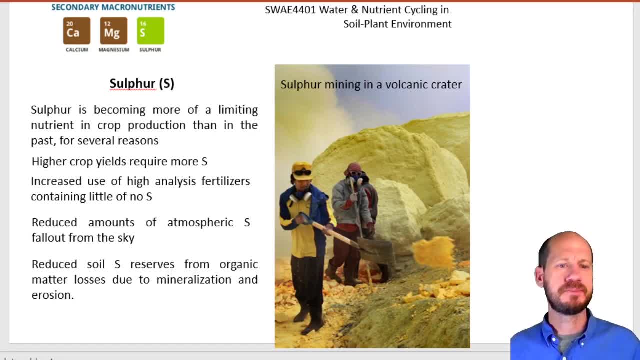 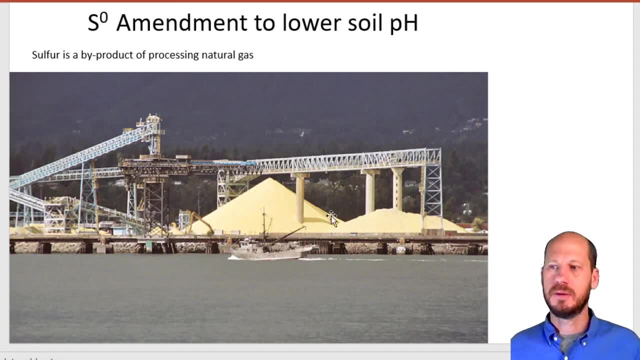 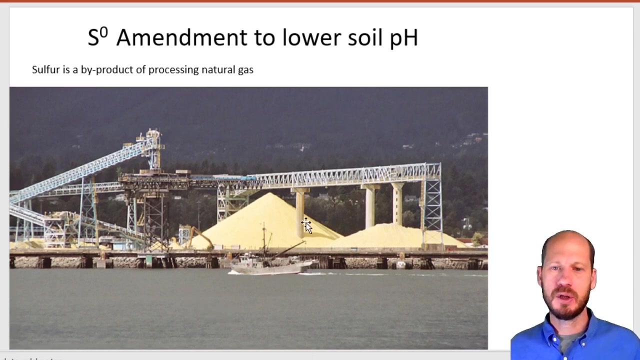 creatures. has this element of sulfur being mined here, but lately this is coming from the oil industry. yeah, the production of gas. there is a process, a microbial process, that is used for removing hydrogen sulfide from the gas, and then what you end up is a lot of elemental sulfur, and this is being used now as an 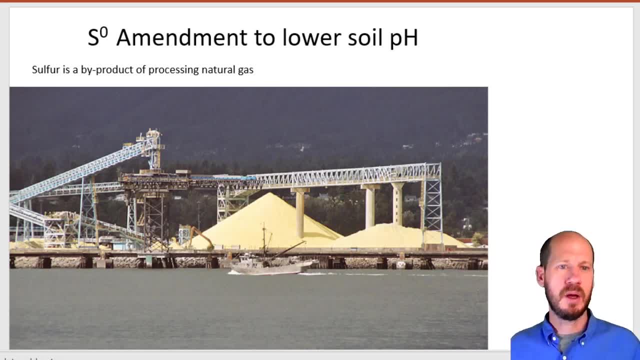 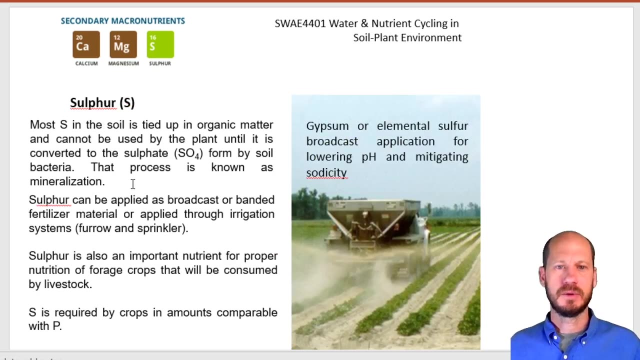 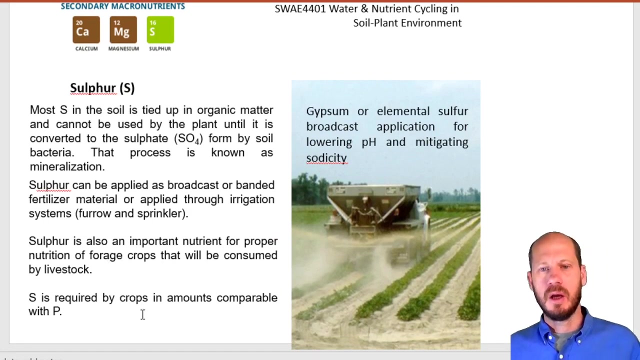 amendment for soils for different reasons, mainly for supplying sulfur to plant nutrition, but also for acidifying soils when the conditions are highly alkaline. all right, so so you have that sulfur is mainly locked in organic matter. when you want to correct sulfur, usually gypsum is the form of sulfur that you apply to soils: calcium sulfate. 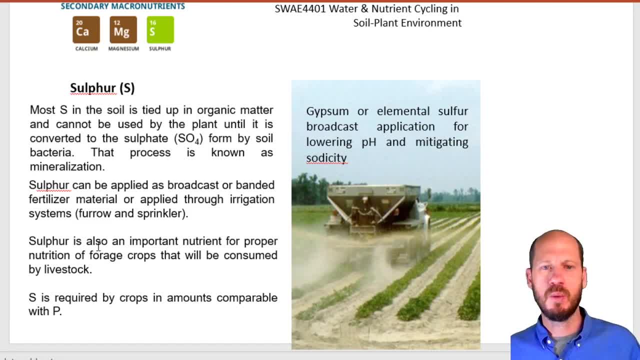 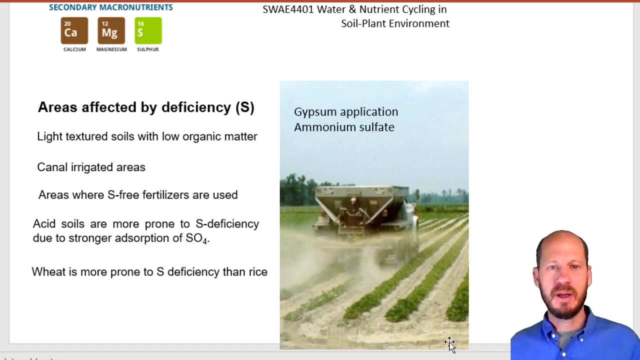 that's about a source of calcium and sulfur. gypsum will not change heavily the pH as lime would, but it will be a source of nutrients. it will be a good source of calcium also to neutralize the negative effect of sodium. if you have high salinity, normally you will have that soils which are very sandy and when 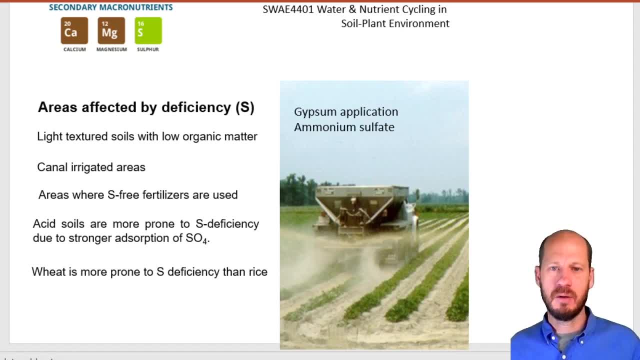 they're irrigated by flooding, like the case of date palms in Oman, for example, you might have sulfur deficiency if you have excessive washing of the soil and the soils are very sandy. you will, but you might end up with sulfur deficiency in these situations. normally, this is well counteract in Oman. 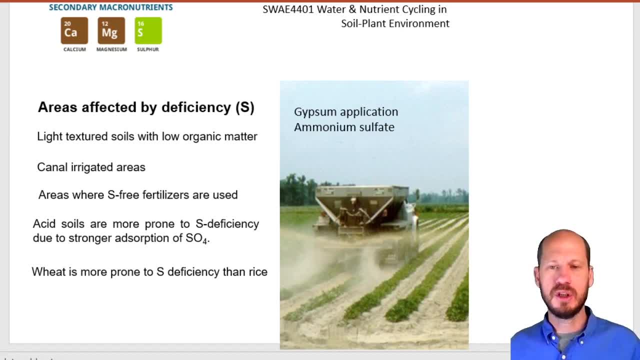 by using a lot of manures, so traditional date palms. in Oman they, although they are doing these flooding irrigation constantly and They have sometimes a high leaching of the soils, but they are usually using a lot of manures on this soil so that these manures are a good supply of sulfur.